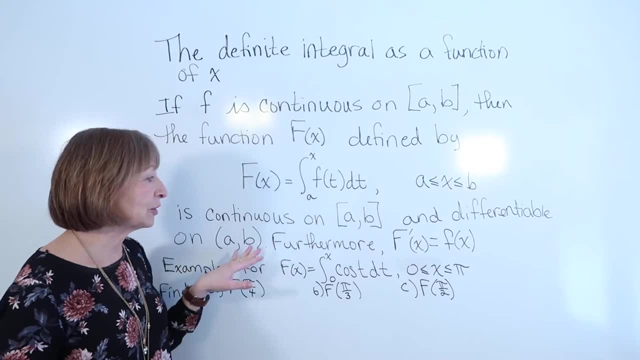 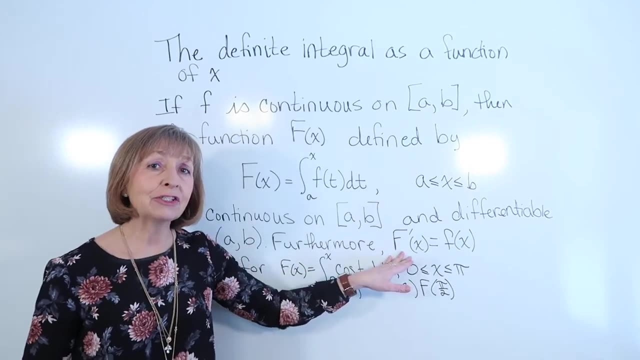 closed interval. So if f is a continuous function on a closed interval, then the function capital F of x is defined by the integral from a to b and it's differentiable on the open interval between a and b. And furthermore, it's true that if you take the derivative of this function, that's defined as an. 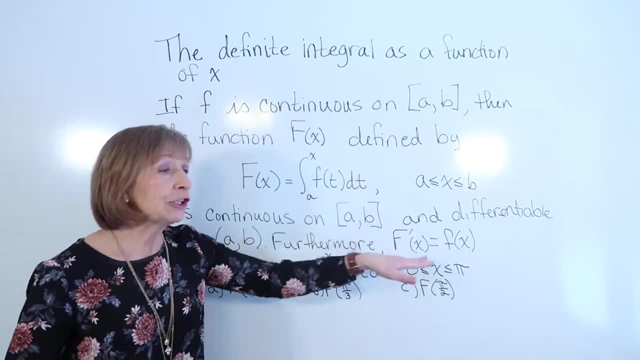 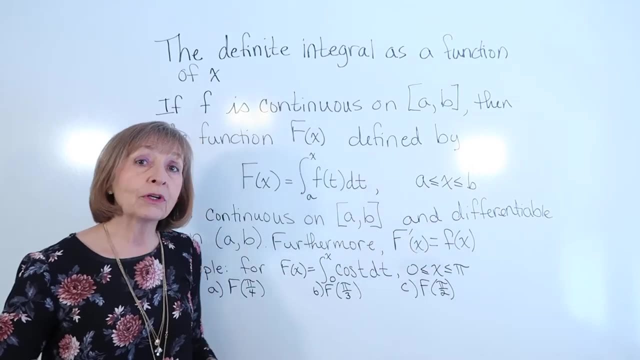 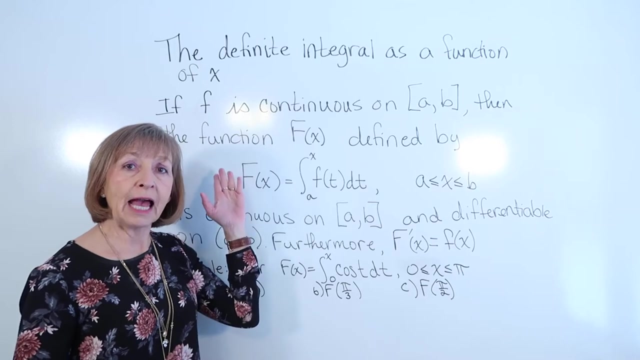 integral from a to x of f of t dt. you actually get this function in x. So what we're going to do here in looking at this is the first thing we're going to do is just look at some of these functions, examples where we have our capital F of X function defined for a specific 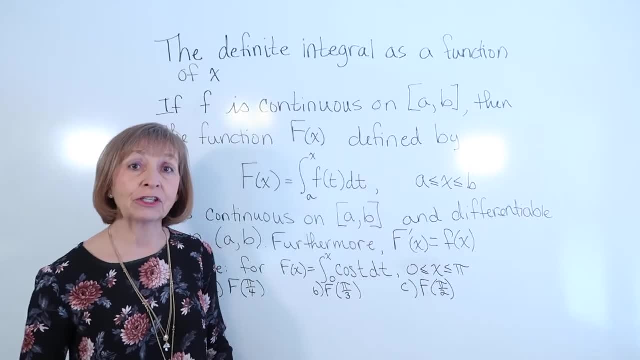 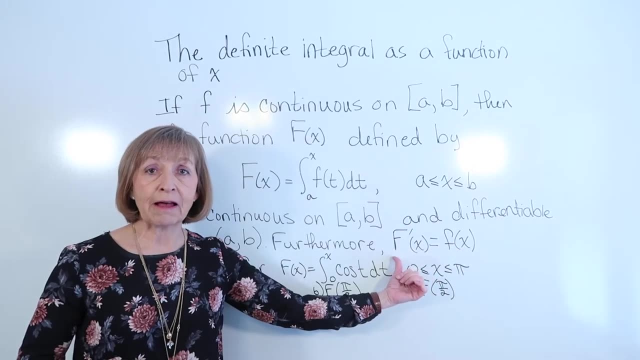 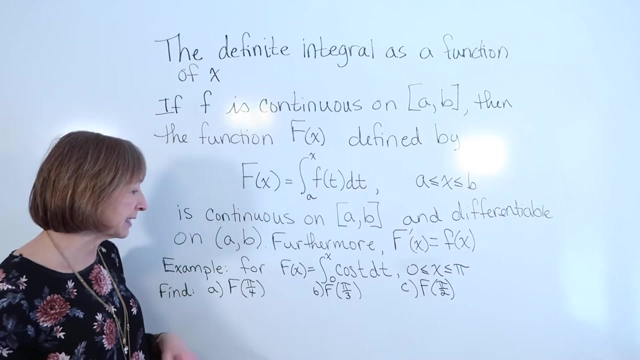 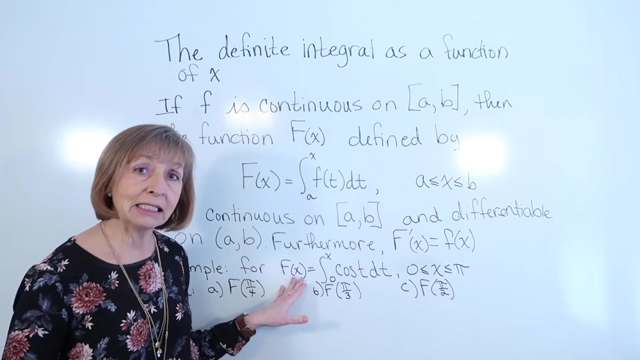 function evaluated at some values. but then we're going to look at what this other part says, that the derivative of our capital F of X function is actually going to be our integrand function of X. so let's get started with that. so here our function, capital F of X for this example, is defined to be the integral. 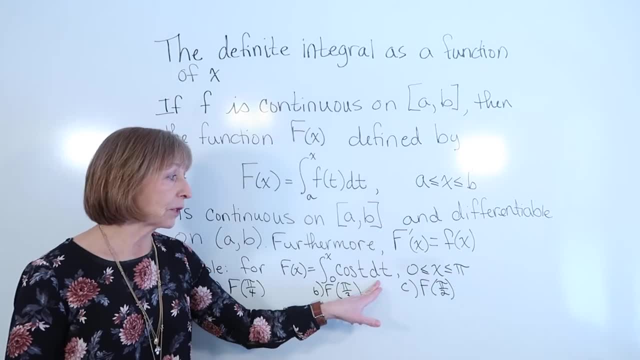 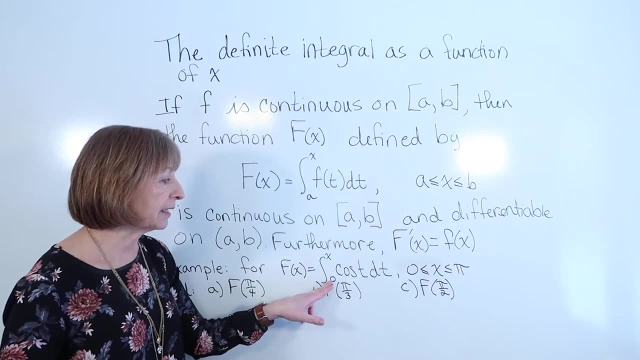 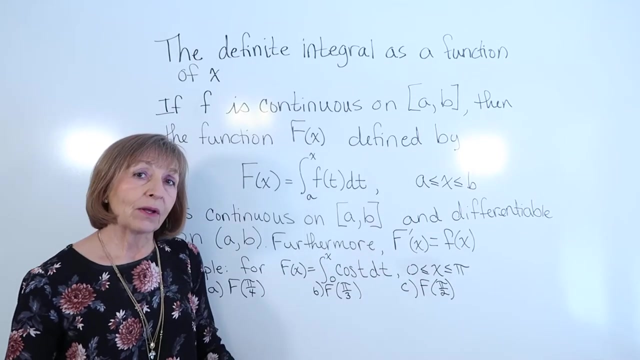 from 0 to X of cosine t dt, where X is a value that I pick somewhere between 0 and pi. so notice my lower limit of integration. here is the start of the interval for which the X's can be picked. now we could go through and generally. 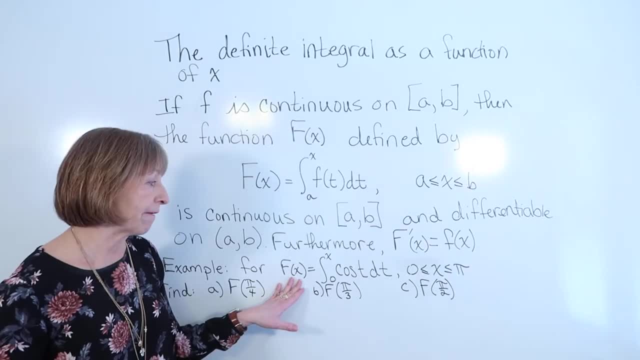 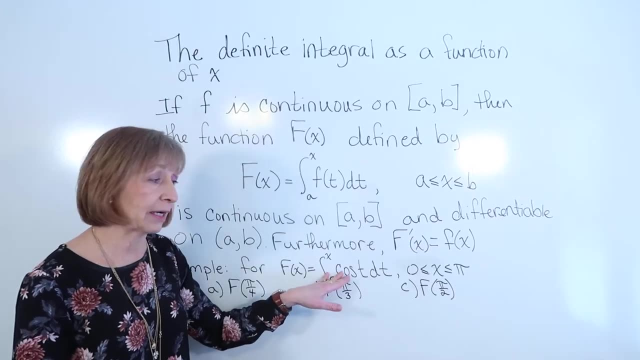 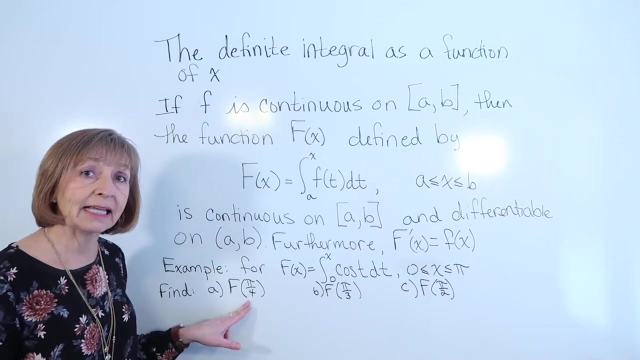 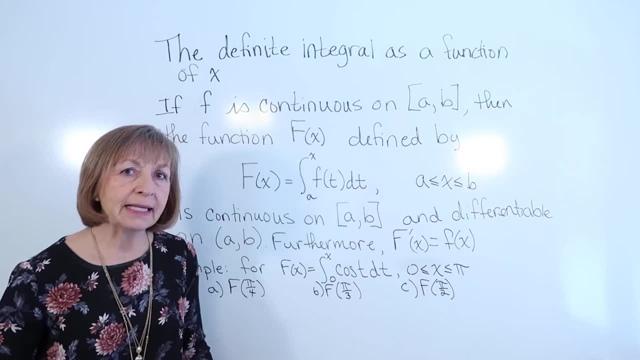 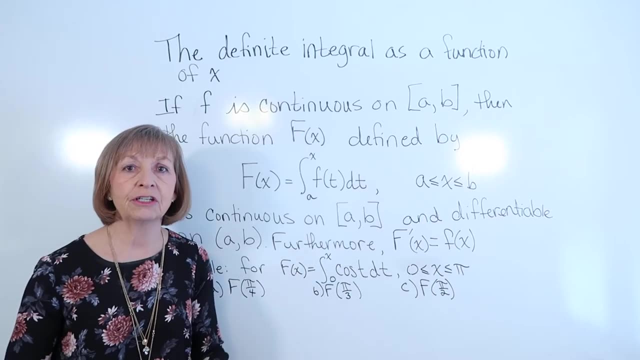 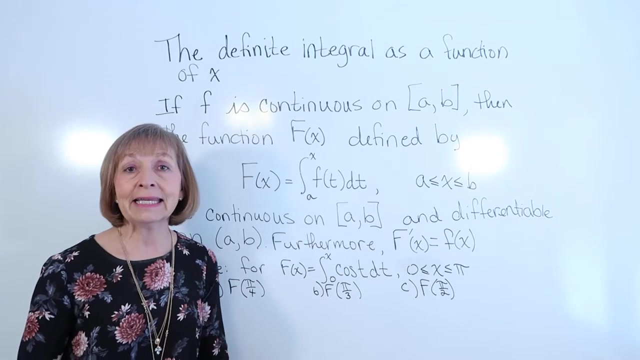 thing. so what I'm going to do, just to prove that point, is I'm going to evaluate the first one by taking out the X in the definition of my capital F of X function and then getting that value out and then after that seeing how we could get our general equation for that function and then go from there. so 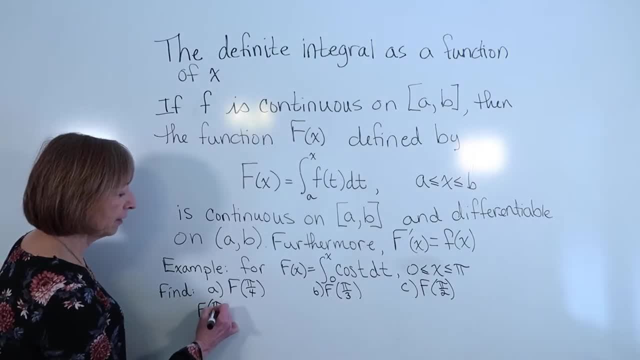 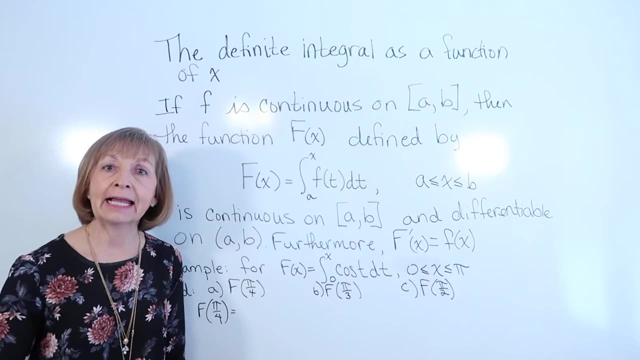 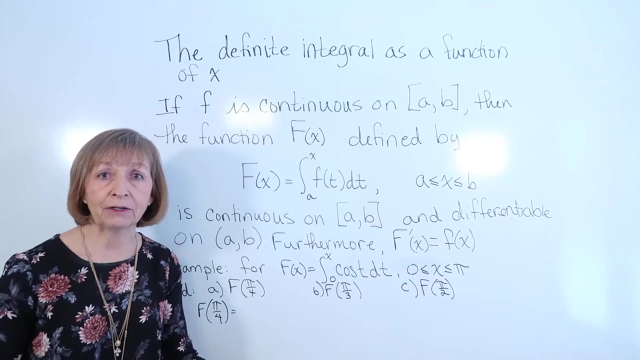 here my capital F of pi over 4. well, think about any other time that you are asked to evaluate a function at an input value, and you've been doing that for a long time. right, you go and you find your variable, your independent variable of your function. take out that variable and replace it with the expression or: 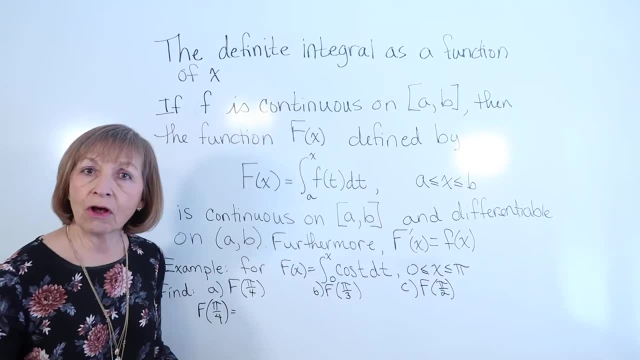 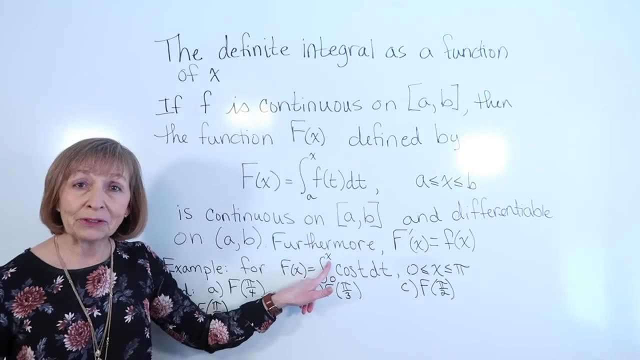 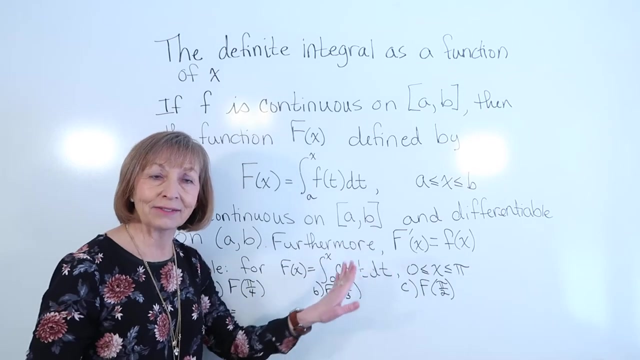 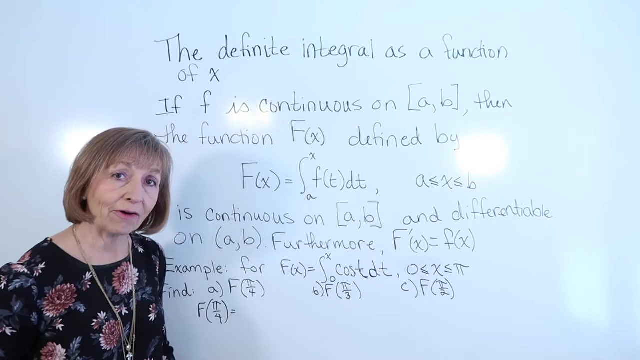 number that you're supposed to evaluate it at, and that's all we want to do here. it's just that it's a little bit uncomfortable for us at first, because here my variable of my function is actually an endpoint of the integral, it's not the variable that is in the integrand itself. 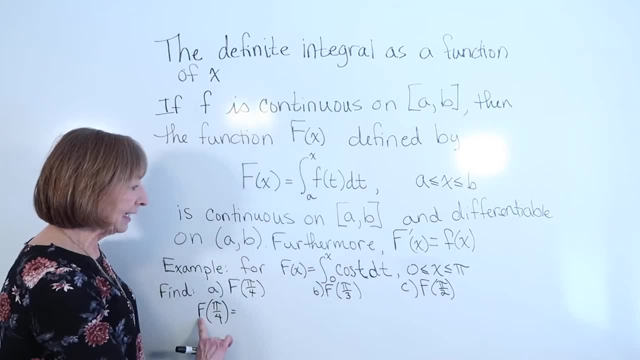 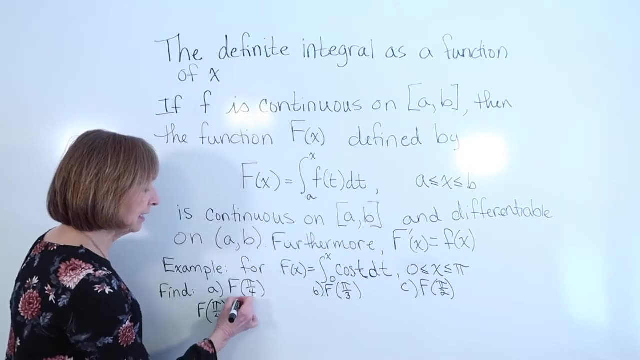 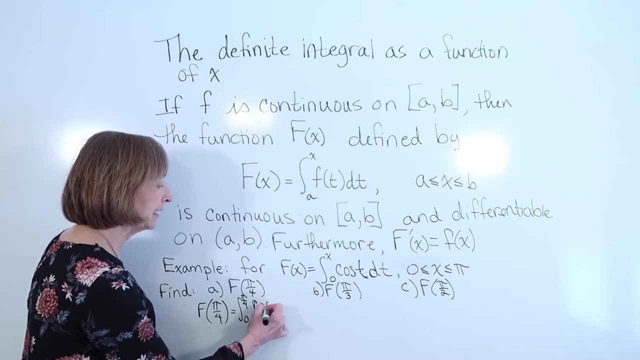 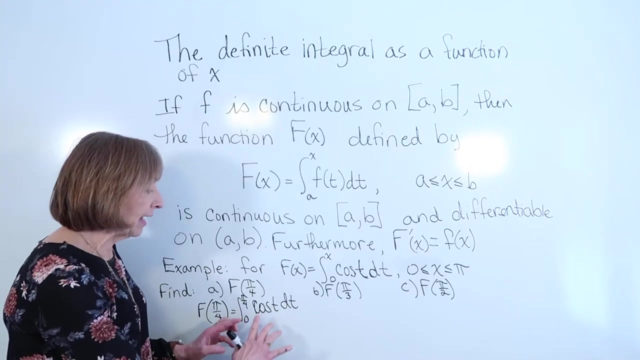 so, when I look at finding capital F of pi over 4, well, this is capital F of X, and X is there. so this is going to be the integral from zero to pi over four of my cosine of Dt. so then this: remember now that I have my definite integral. 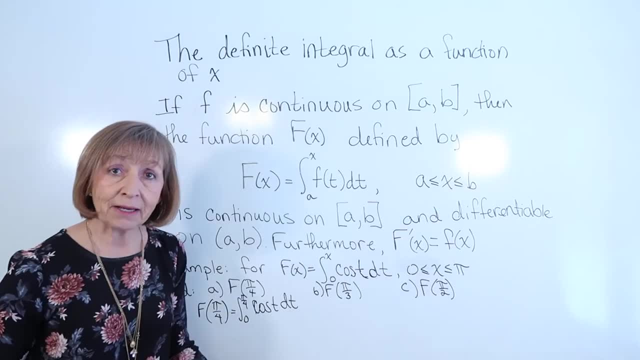 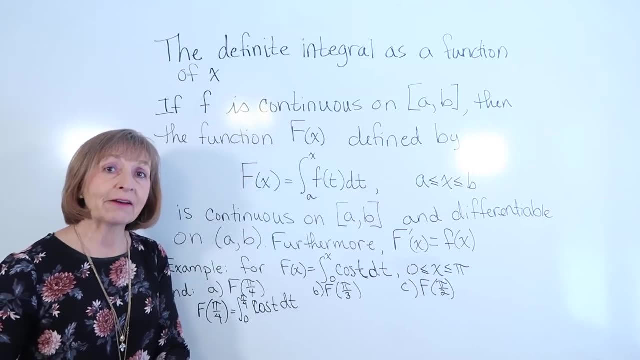 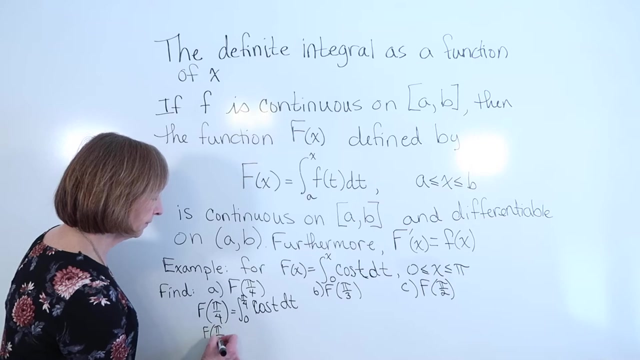 from a number to a number of a function. that's going to be a number. I can use my fundamental theorem of calculus from helping me evaluate a definite integral here and that will give me my value out. So my capital F of pi over 4, we're going to get by finding an antiderivative of cosine t. 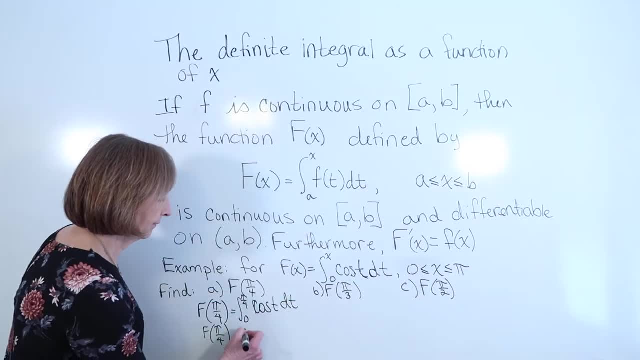 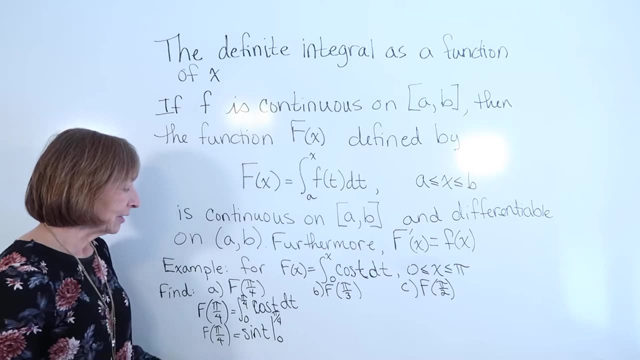 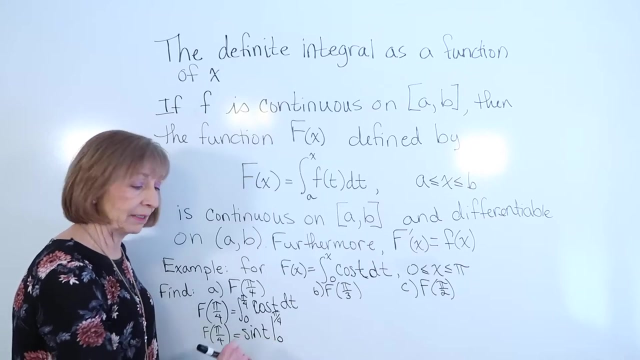 An antiderivative of cosine t is sine t. Evaluate that from 0 to pi over 4.. And then, remember, you evaluate it by putting in the upper limit of integration to the variable minus the lower limit of integration to the variable. So my F of pi over 4 is sine of pi over 4 minus the sine of 0.. 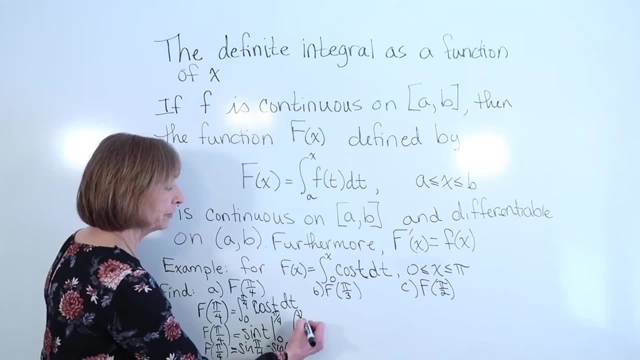 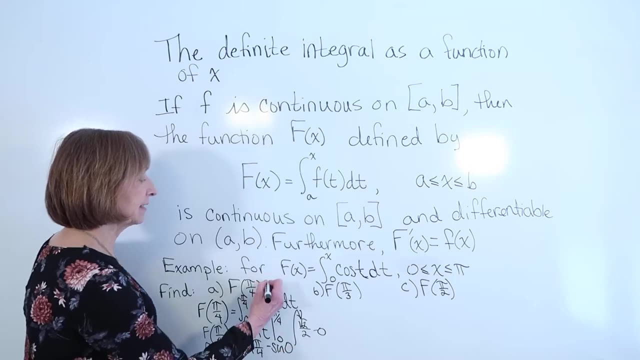 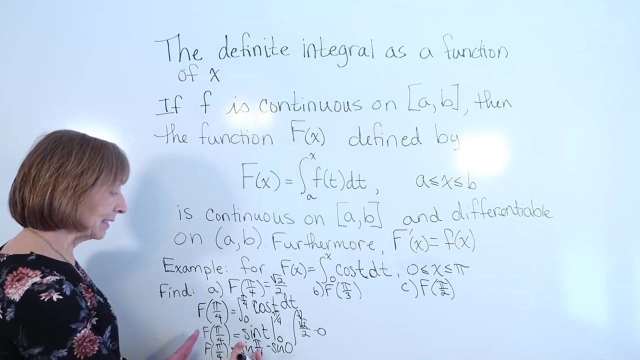 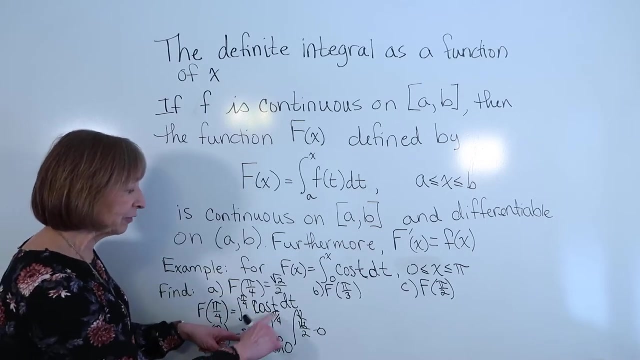 And the sine of pi over 4 is the square root of 2 over 2.. The sine of 0 is 0.. So I get for this that that's the square root of 2 over 2.. So that way of evaluating my function would require me to do this process of finding my antiderivative. 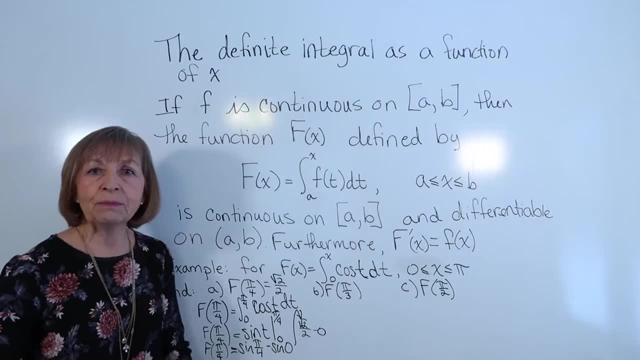 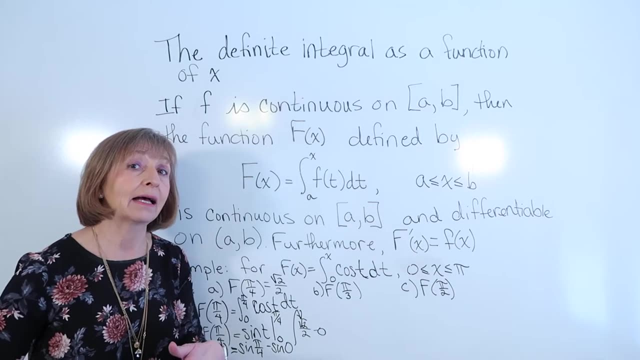 plugging in the numbers and then evaluating it out. It would be like if I were working with an equation of a line and I had several different x inputs and I want to find the y outputs but I don't have. I don't have it solved for y. 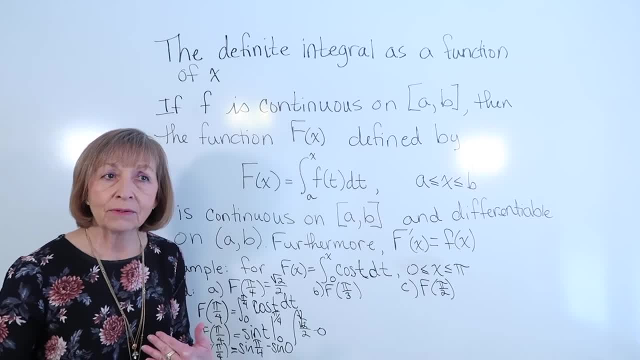 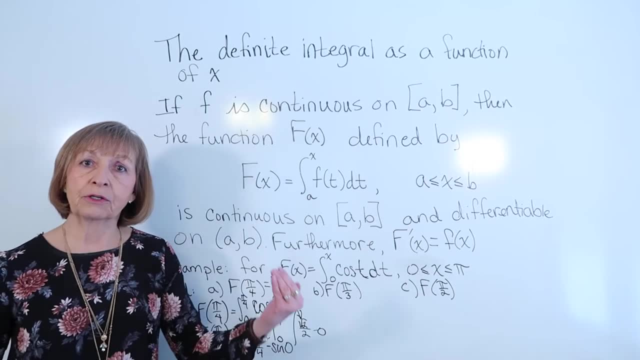 So every single time I would have to resolve it for y. That would take a lot of time. It would give me the right answers, But a better thing to do would have been to solve the algebraic equation for y in the first place. 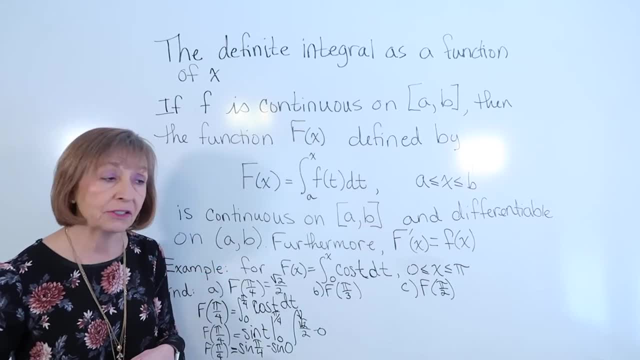 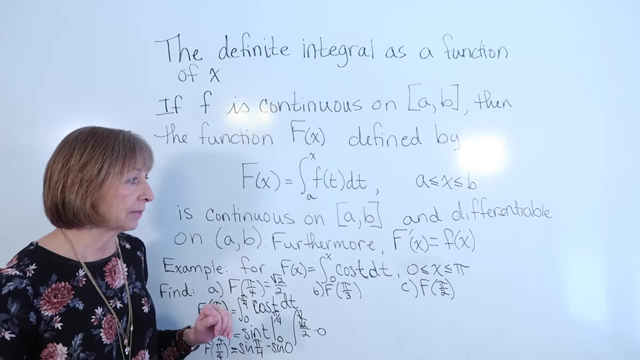 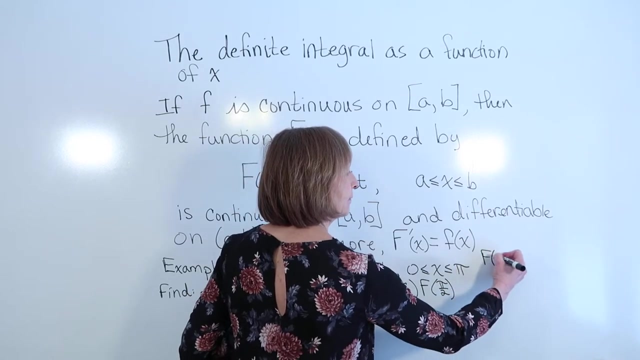 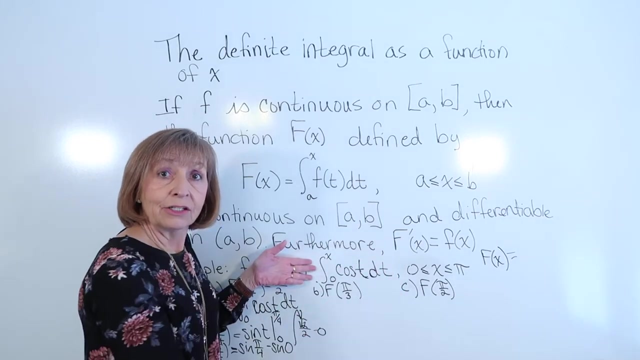 and then just plug in the varied x's that we want to use. So here, instead of plugging it in and integrating it new each time, what we could do is take and look at this capital F, F of x and then think about how we would integrate this using the work with the fundamental theorem of calculus. 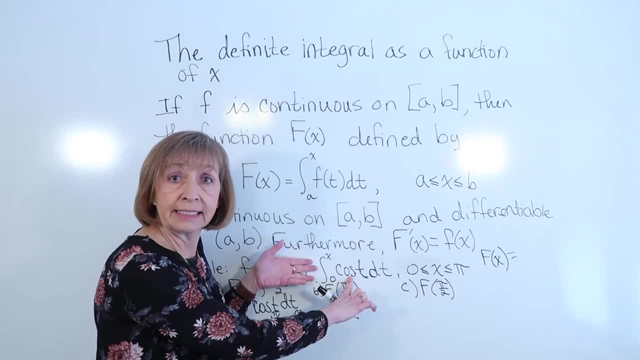 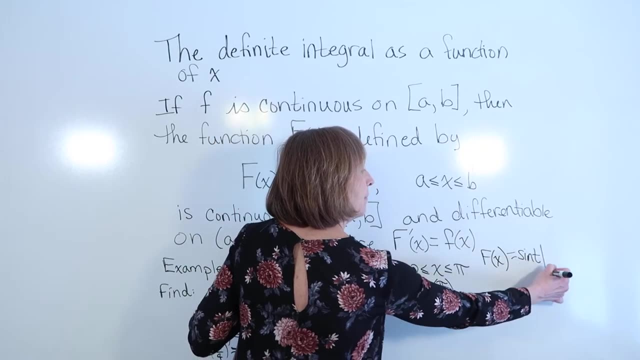 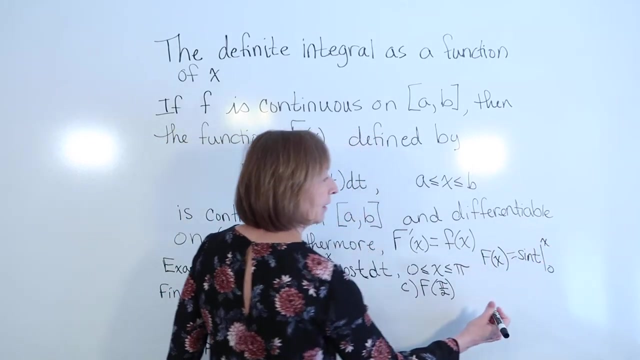 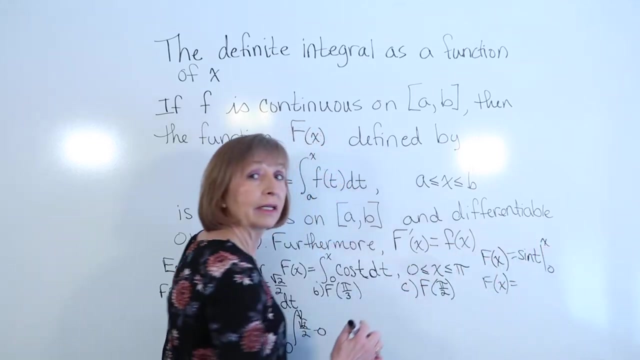 So we are going to find an antiderivative of cosine t. An antiderivative of cosine t is sine t, But I'm going to evaluate that from 0 to x. So then we take out the variable and replace it with the upper limit of integration. 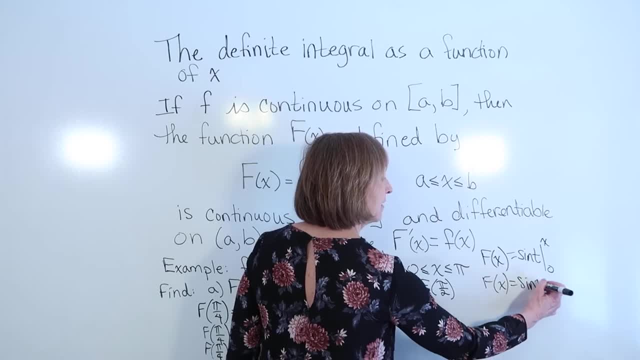 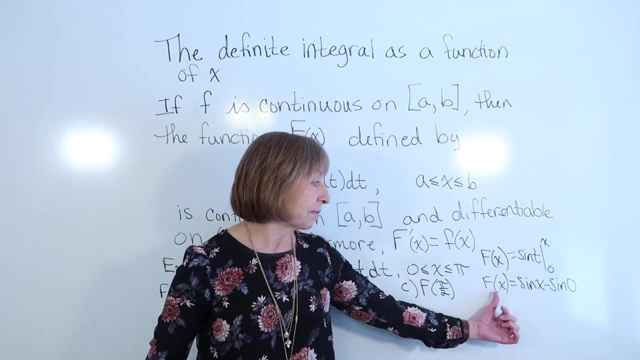 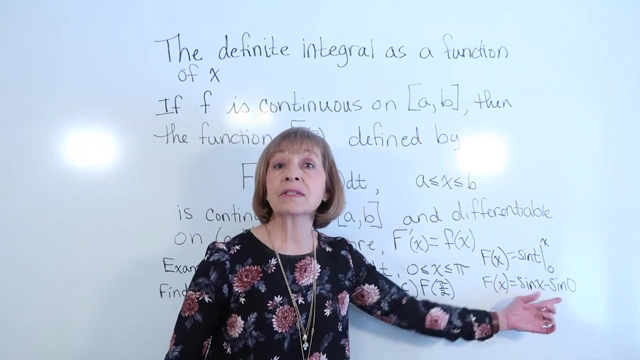 So take out the t and put in the x, I have sine x minus the sine of 0, putting in the lower limit of integration, And my capital F of x for this particular function is sine x minus. Well, the sine of 0 is 0.. 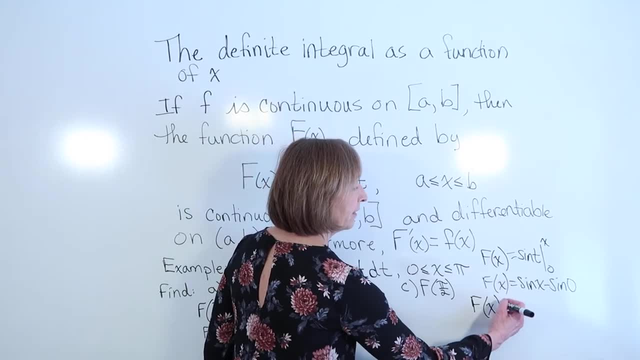 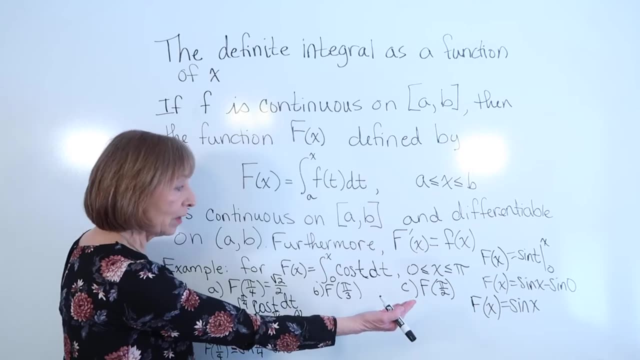 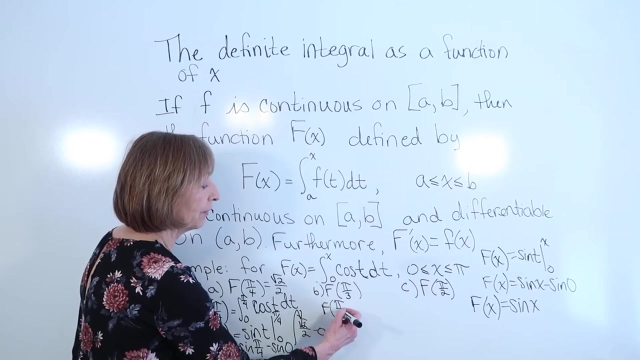 So I just get that this capital F of x function is just the sine of x. So since I did all that work once, now I can go ahead and say: well, that means for F of pi over 3,. I'm just going to go and evaluate the sine of pi over 3.. 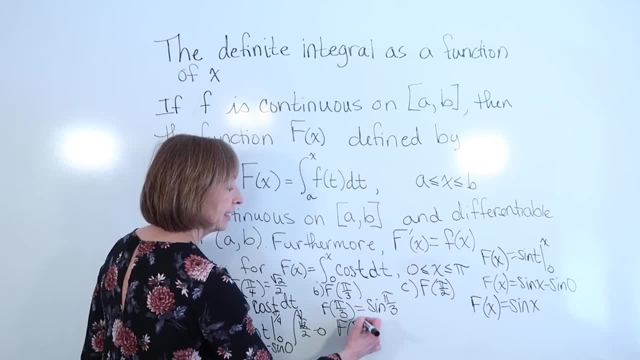 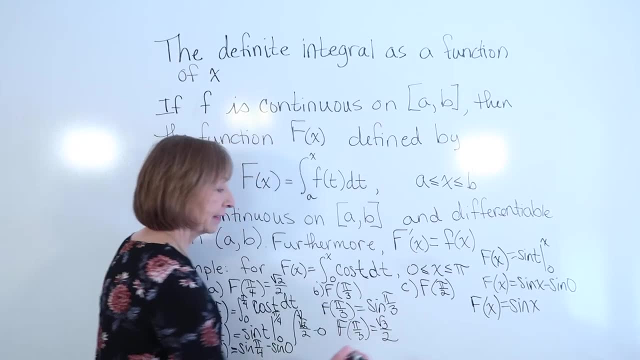 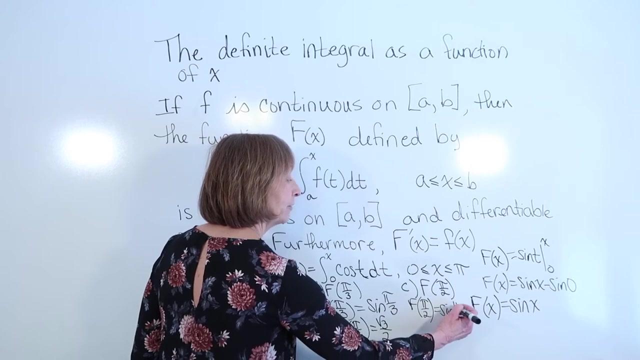 So my capital F of pi over 3. Is equal to. Well, the sine of pi over 3 is the square root of 3 over 2.. And then my capital F of pi over 2 is equal to the sine of pi over 2.. 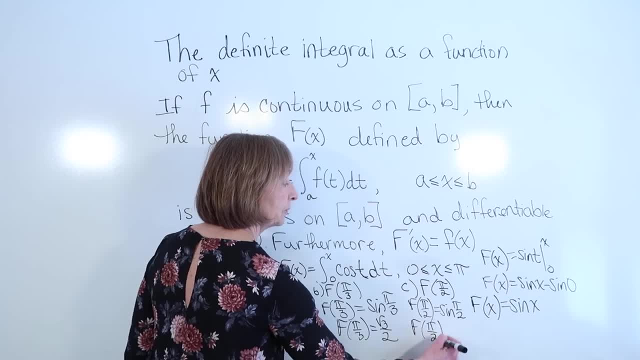 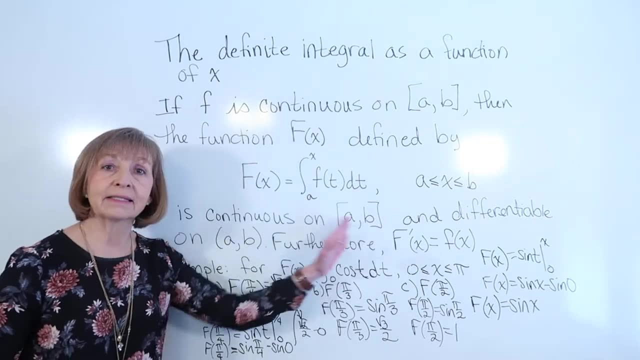 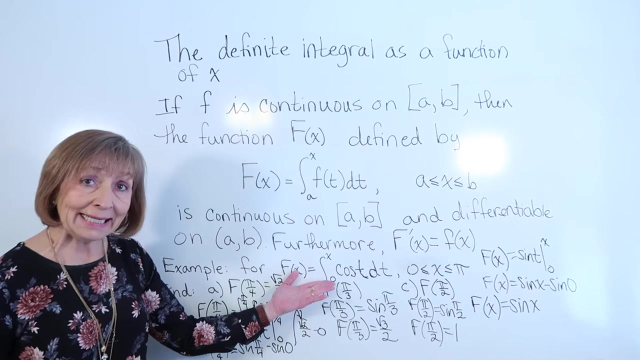 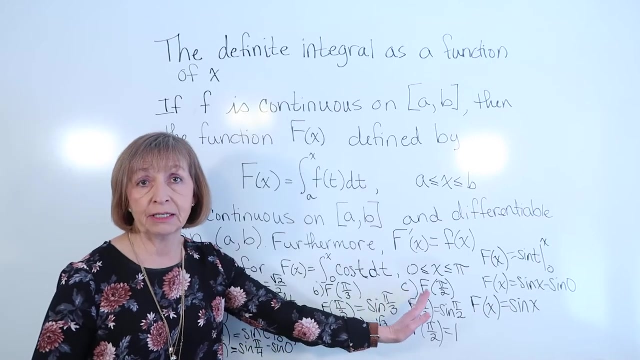 And the sine of pi over 2 is 1.. So working through what this definition of my capital F of x is equal to. So working through what this definition of my capital F of x is equal to, and getting its equation actually aided in being able to evaluate it at different input values easier, 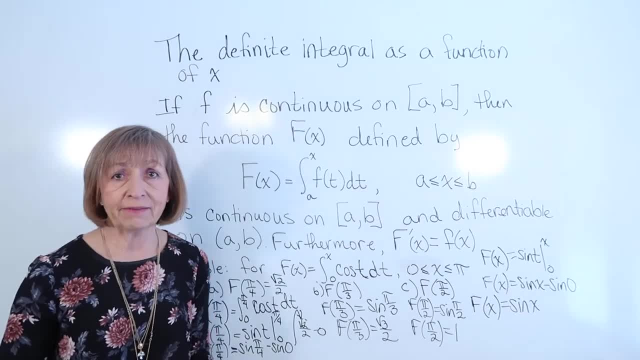 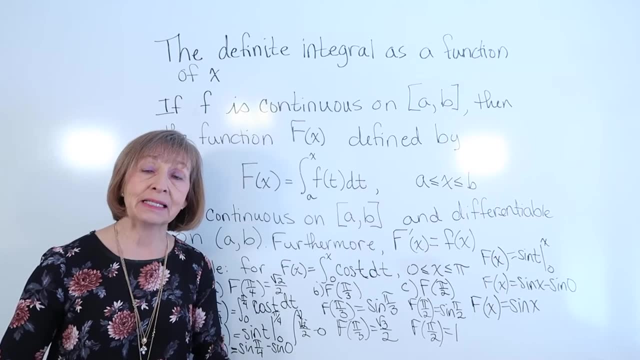 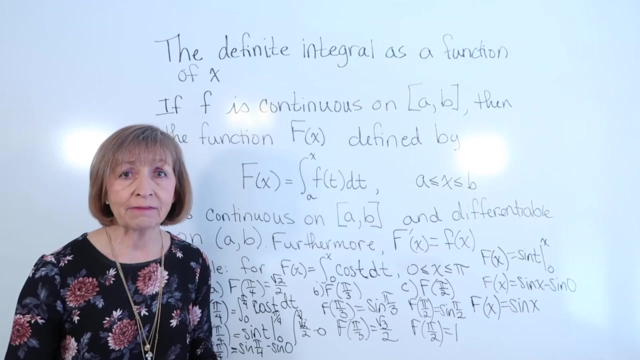 What if you know that you have a continuous function on a closed interval and your function capital, F of x is defined to be the integral from a to x of f, of t, dt, and you weren't wanting to evaluate it, and you weren't wanting to evaluate it at values? 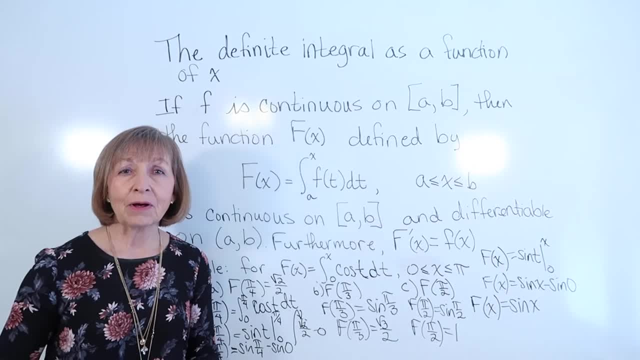 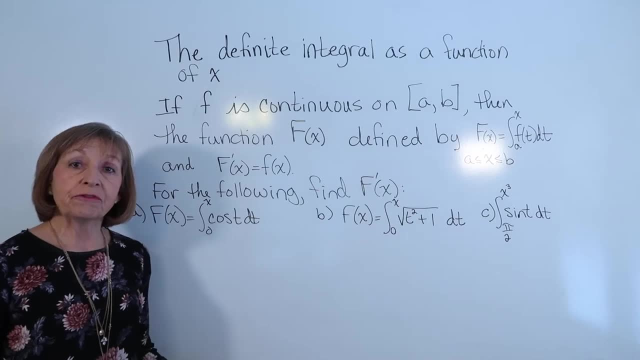 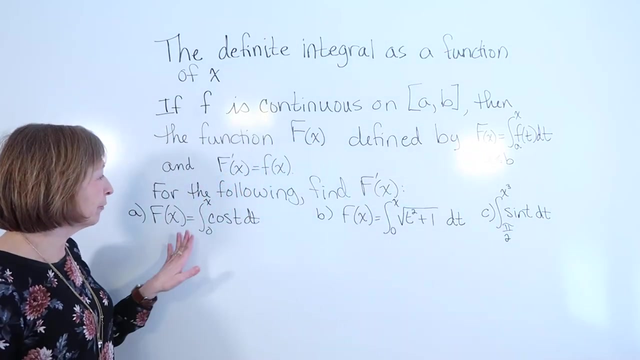 you actually wanted to find the derivative of it. Well, that's what we're going to do next. So let's look at what if they ask us to find the derivative of our function that is defined in this manner. So first of all, I have my capital. F of x is defined to be the integral from 0 to x of cosine t dt. 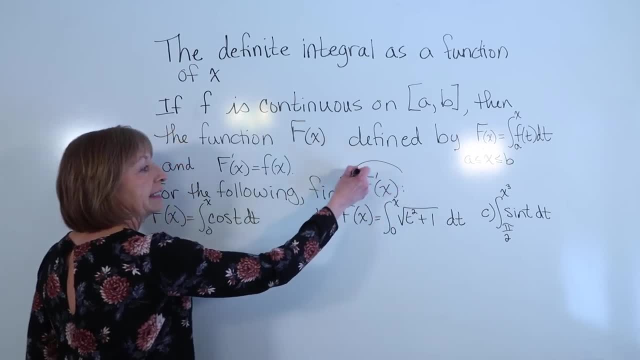 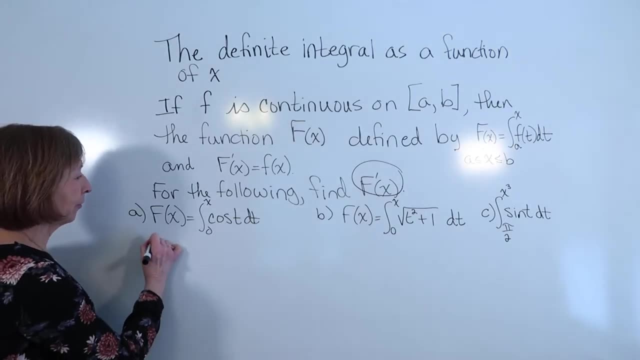 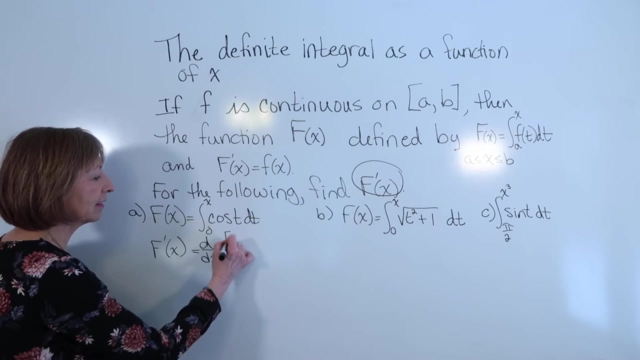 and in the direction it says find f and in the direction it says find f of x, is defined to be the integral from 0 to x of cosine t dt. So when I think about asking me to find f, prime of x, they want me to find the derivative, with respect to x, of this integral from 0 to x of cosine t dt. 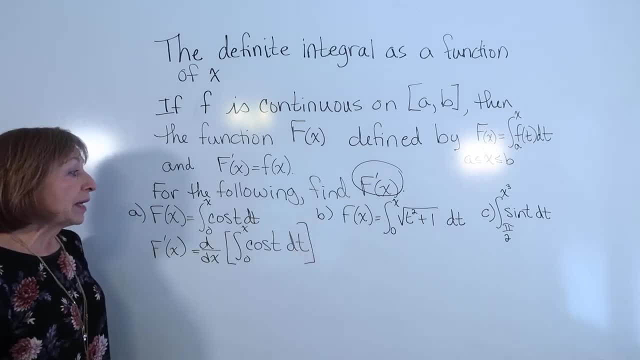 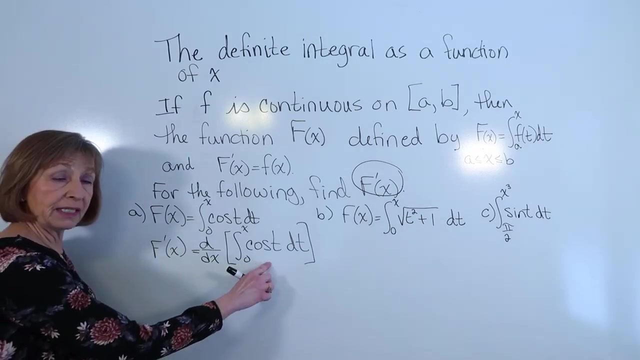 Now, when I'm looking at how this is defined, I have to make sure that I have my lower limit of integration be my, and my variable be at the upper limit of integration. Now, what I'm going to do with this is work from the inside out. 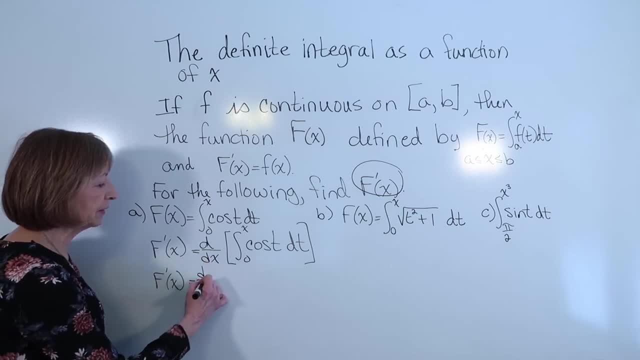 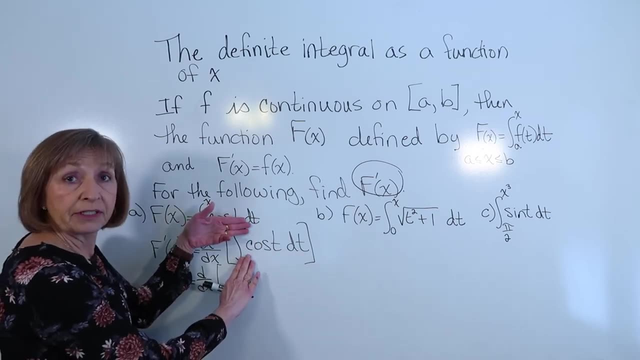 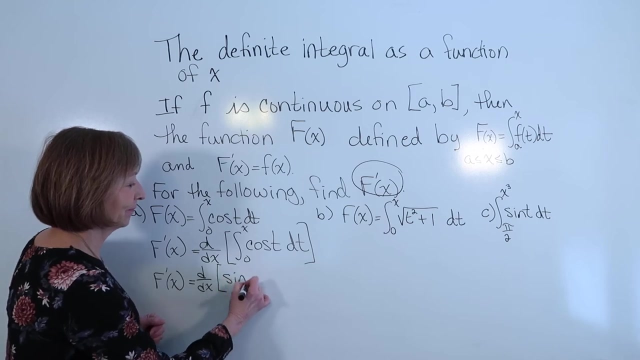 So my capital F of x is equal to the derivative with respect to x of. well, the integral from 0 to x of cosine t dt. Remember we're going to find an antiderivative. An antiderivative of cosine t is sine t. 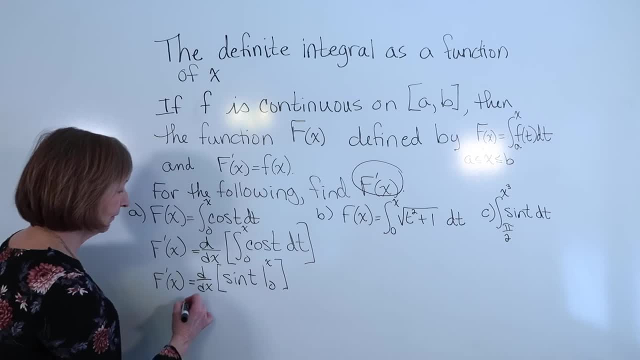 Evaluate that from 0 to x. So then I have it's the derivative, with respect to x, of put in the upper limit of integration, minus put in the lower limit of integration. So this is sine x minus the sine of 0.. 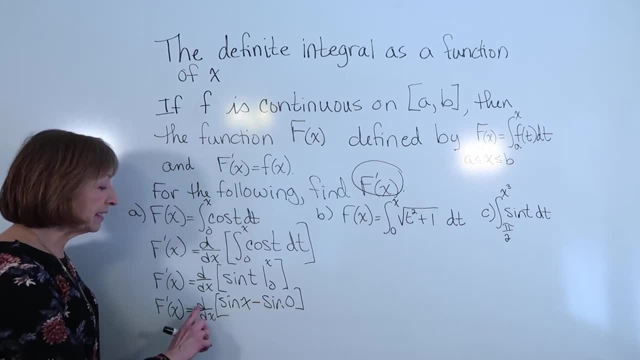 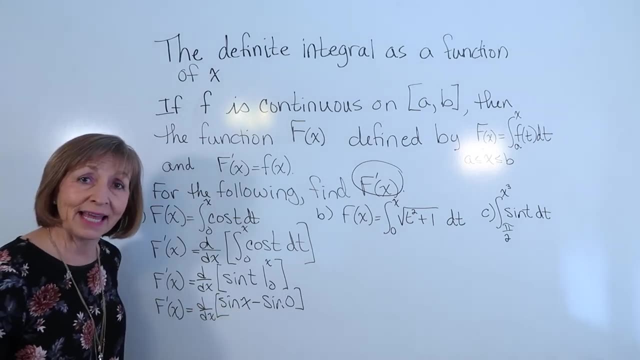 But the sine of 0 is 0.. So this is just the derivative with respect to x of sine of x. The derivative with respect to x of sine of x is 0.. The derivative with respect to x of sine of x is cosine x. 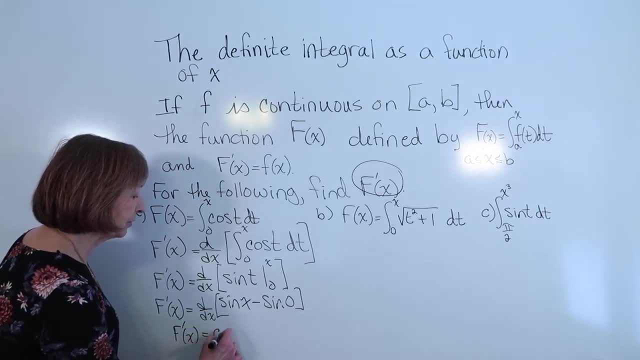 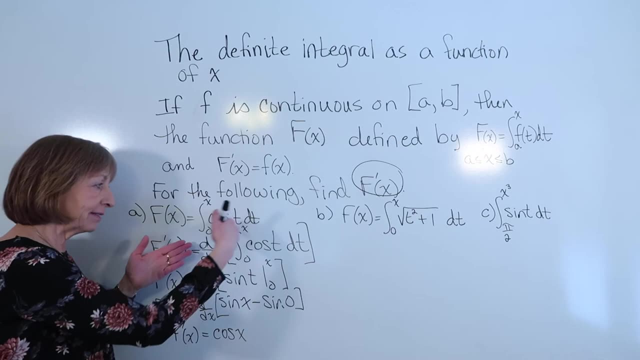 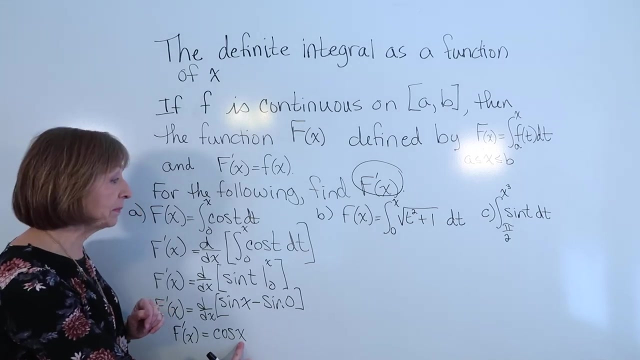 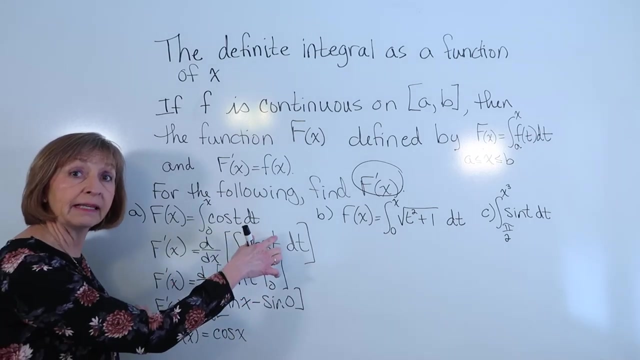 So my capital F prime of x is equal to cosine x, which is what I had in the integrand of the original integral defined function, But now it's in the variable x, because of what happened in our application of working with the definite integral and plugging in the upper limit of integration, which well 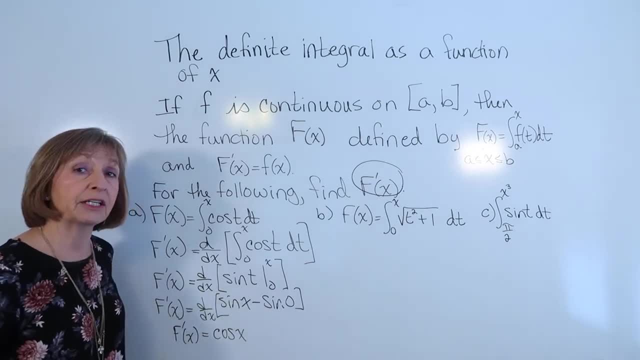 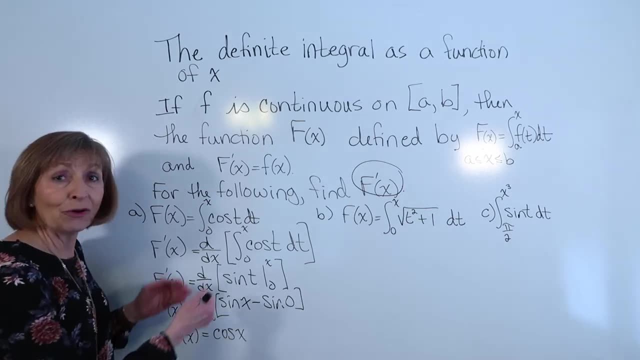 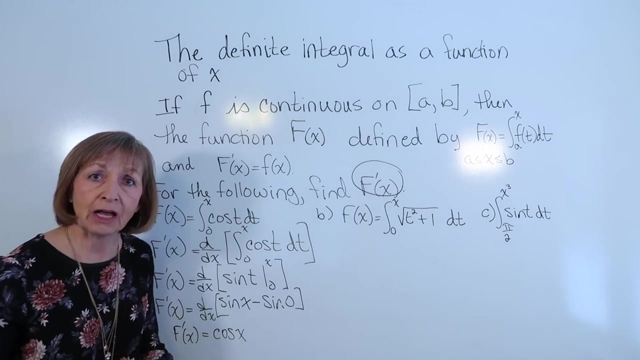 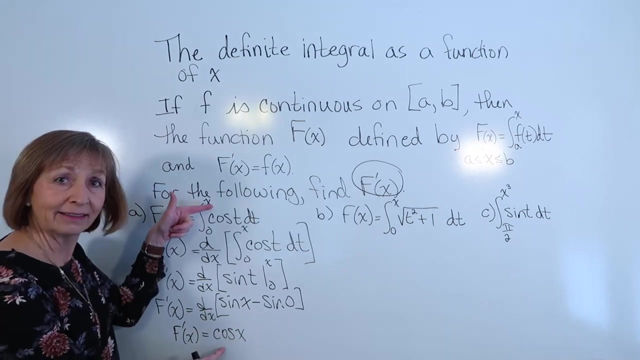 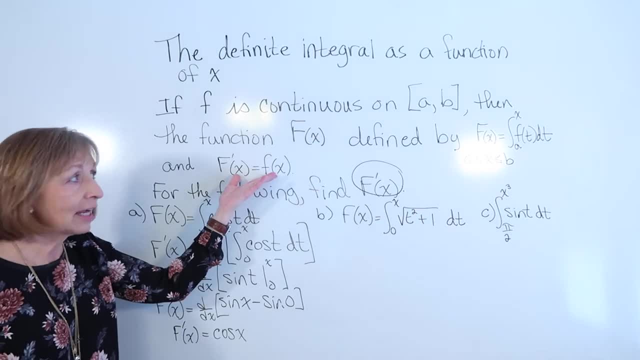 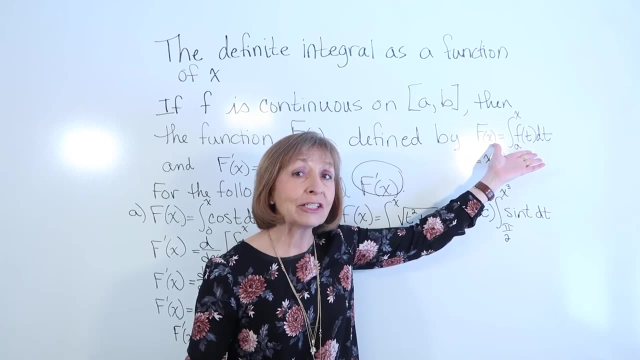 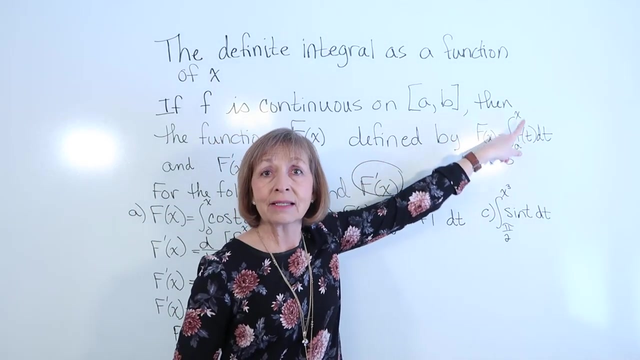 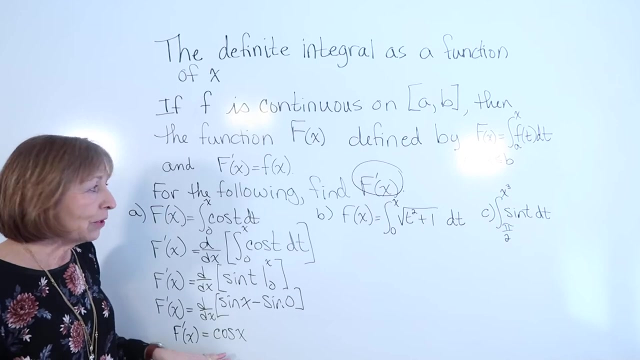 I can say- that's what they were trying to tell me here- that when my function is defined as that type of an integral and I take the derivative of it, I am going to get the function that was in the integrand in that variable x now instead of in the variable t. 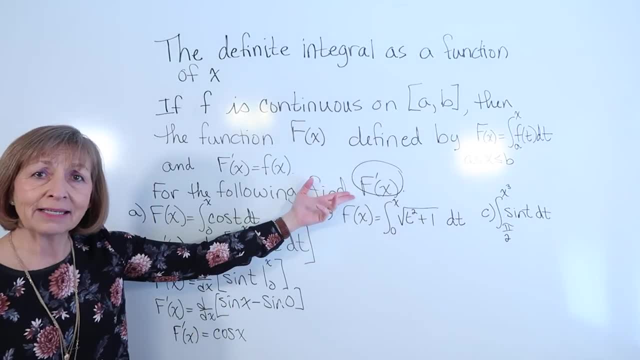 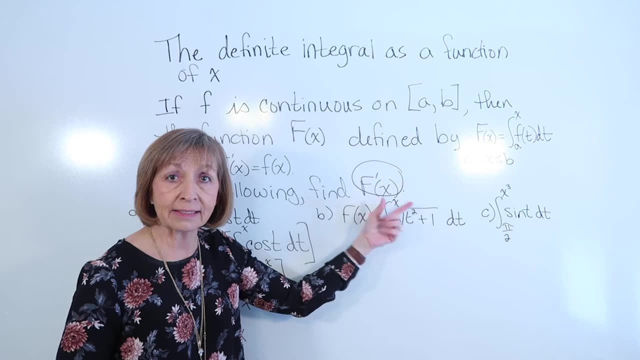 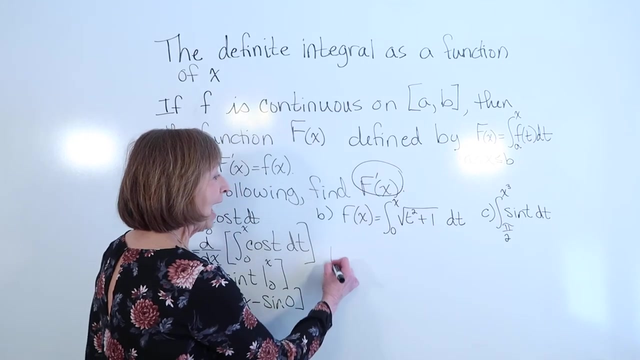 So that's huge, because now, if I'm asked again to find a derivative of this thing, I'm going to use this function that's defined as the integral, from 0 to x, of a continuous function over that interval, which this is. then I don't have to go through all of those other. 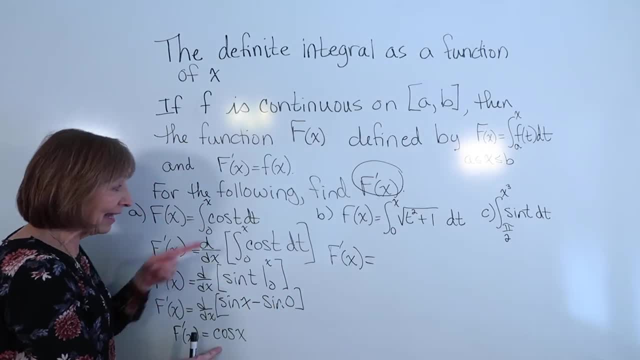 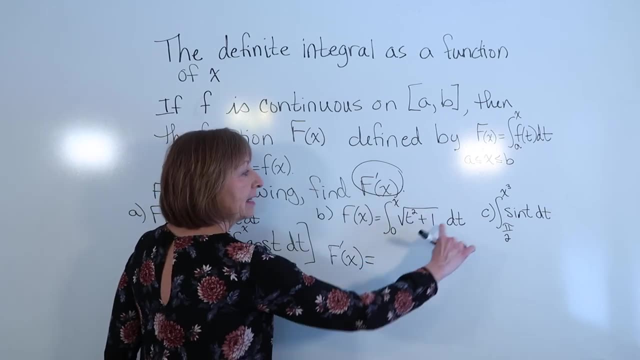 motions, all of this other stuff, to see that I just get that back. I can just jump to the case and say this is just going to be this function, the square root of, but now it'll have that bar, So this is going to always be the other way around. Because whenever I combine these two things again, we're gonna have the same. this is just a different integral. we're not going to either along its own. you have to plug it in. So what happens in lambda get same as this. you're not going to multiply, dash into x. 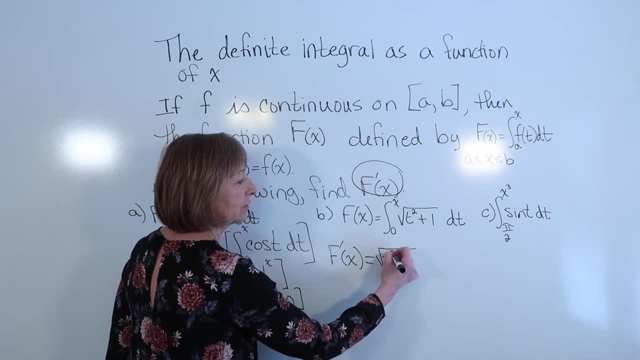 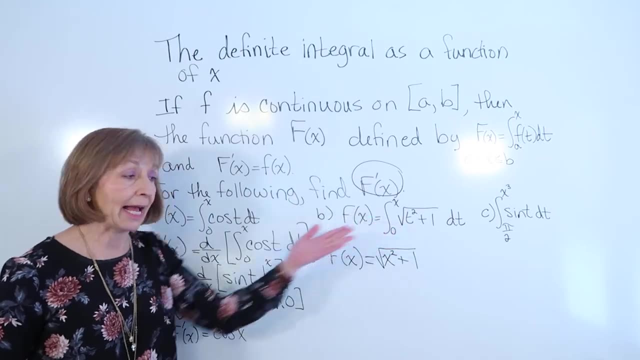 X comes over to y and y same times into x also plays against the previously. it'll have the X's in its place, the square root of x squared plus 1- a much better way of going about this than if I tried to actually do this every time. 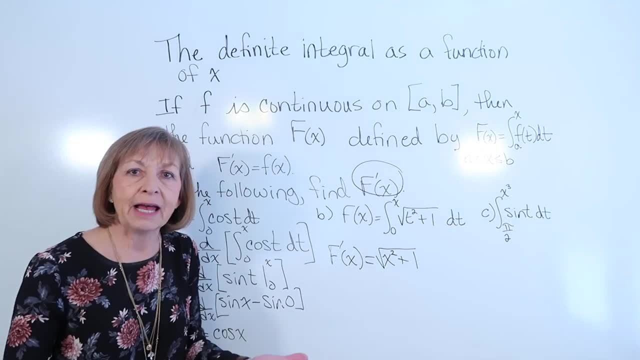 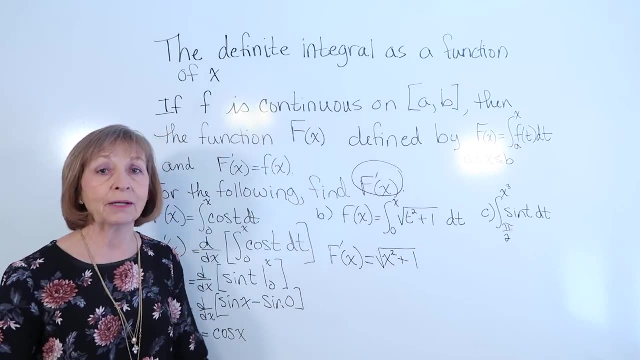 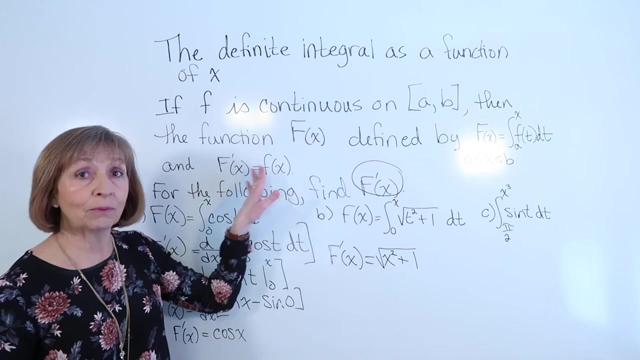 especially if I don't have at my disposal or remember or figure out how to find an antiderivative for that function when I'm just going to differentiate it back and get the original function anyway. so that's really what this helps me with now. this last example that I have actually is: 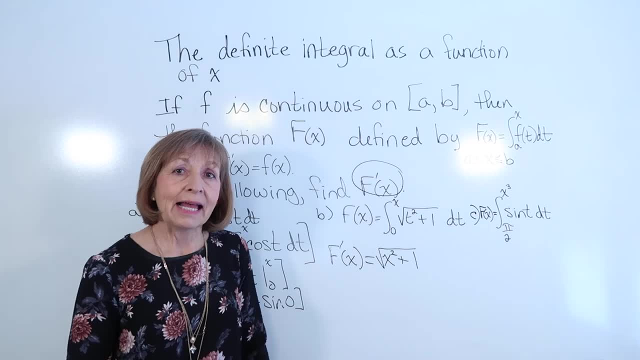 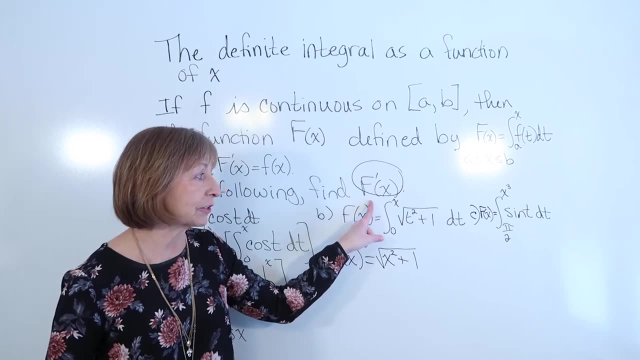 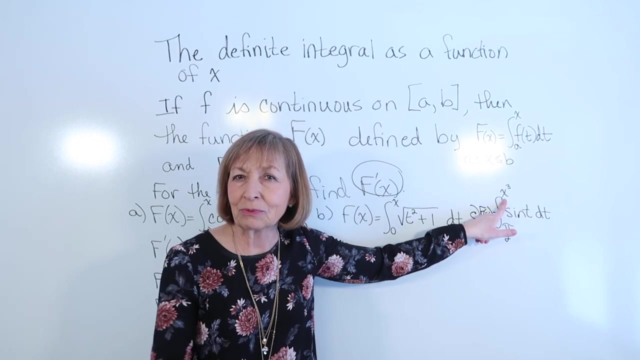 going to use that because sample that I have, it's going to need a little bit more. it's still asking me to find the derivative of that capital F of X function defined as an integral from a constant 2, but it's to an expression in my variables whose derivative is other than 1. and remember when you're 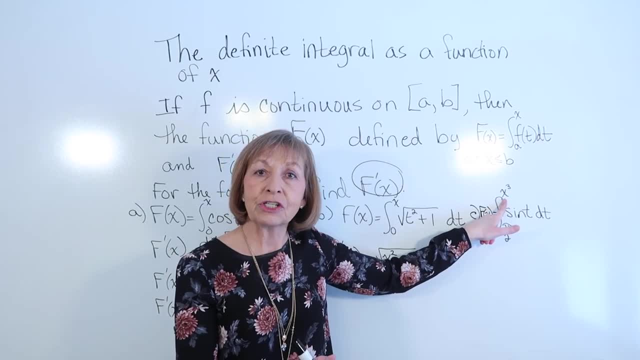 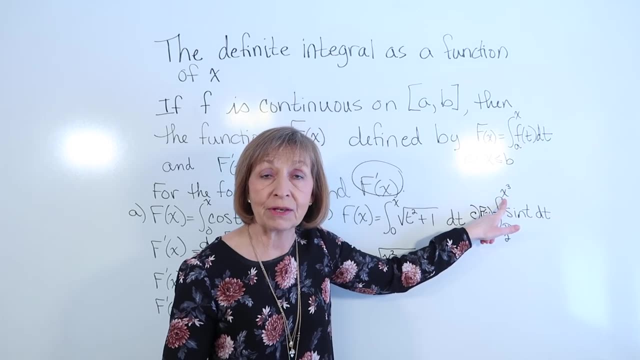 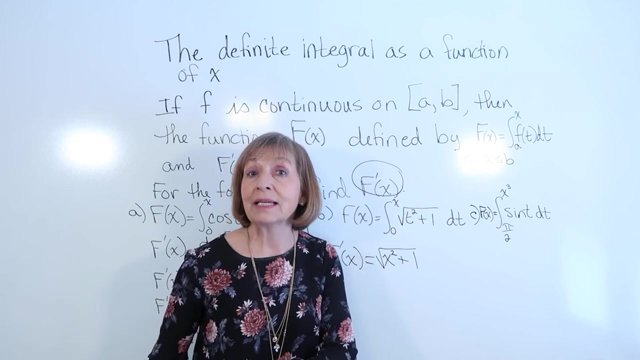 differentiating a function who is a composite function and it's acting on an expression whose derivative is other than 1, then you have to use the chain rule when you differentiate it. so not only do you have to take the derivative of the outside action, keep the inside stuff alone, but then you also have to multiply by the. 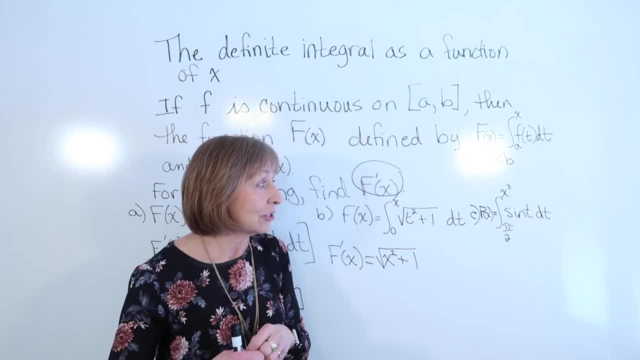 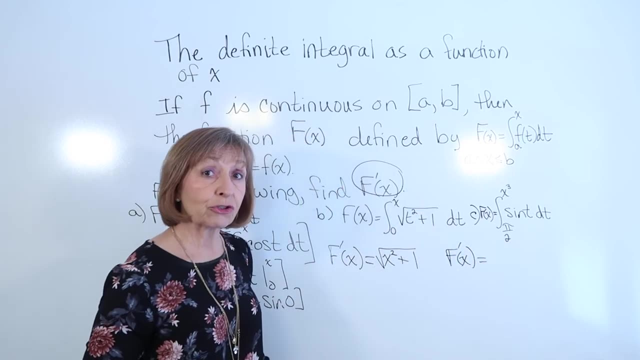 derivative of the inside expression. so when I actually go and do this, step into this step over here, this is these crowd bubbles, and so let's paint the side of the sideboard as the outside shape. so I do 1 by 2 of the clic and 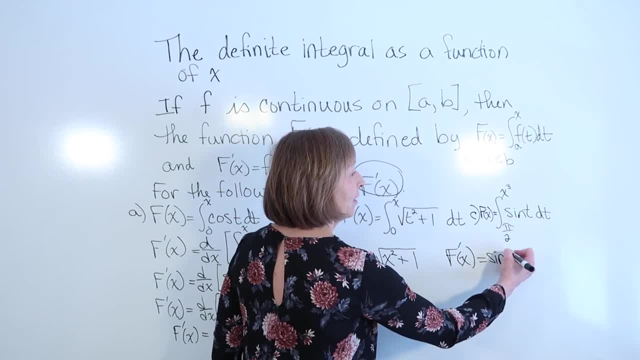 then there are no cursor buttons. but you can see here if the goes out in the corner I can actually take a line tells me. so if I'm drawing curve pattern, go on to Q and it has a value influence and it has this sign of X. Student is. 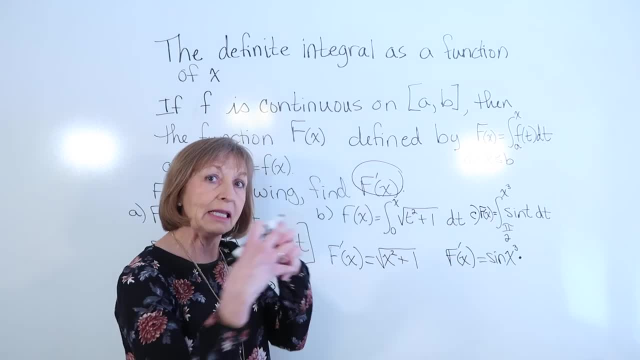 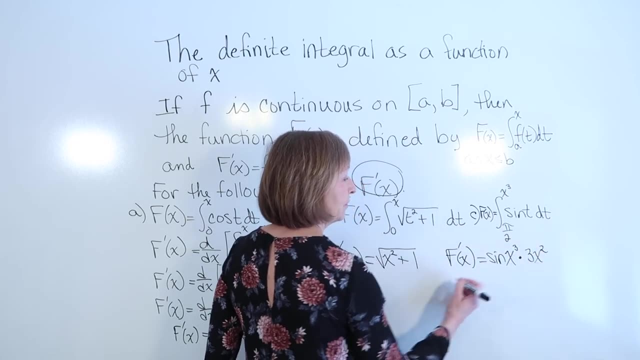 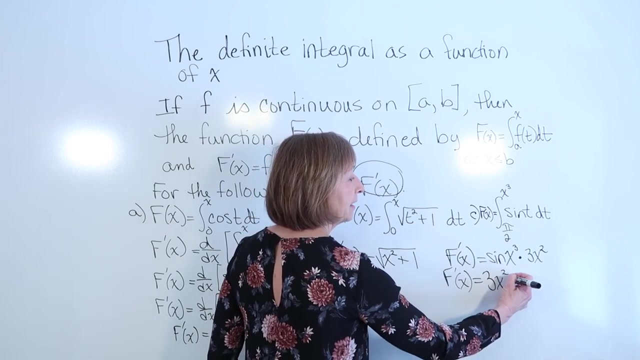 going to know when I'm going to be getting into serve and I just want to reiterate that the state variable is integral from state. despite of greater time, if I am running atcn will be ever greater then Q and cute, because two, two F prime of x, capital F prime of x for this one is 3x squared times the sine of x to. 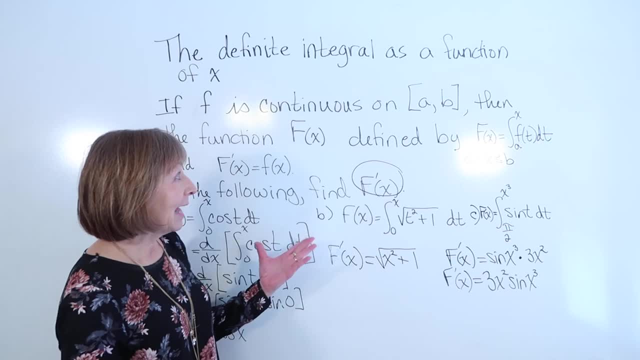 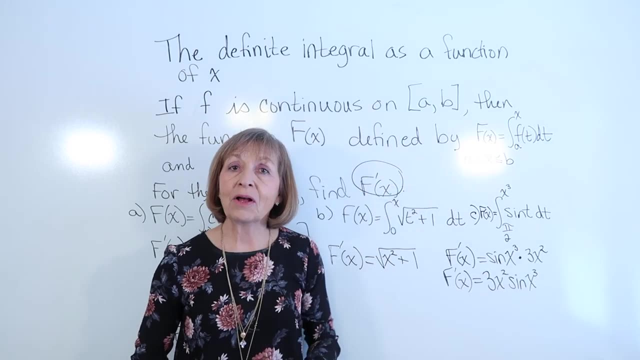 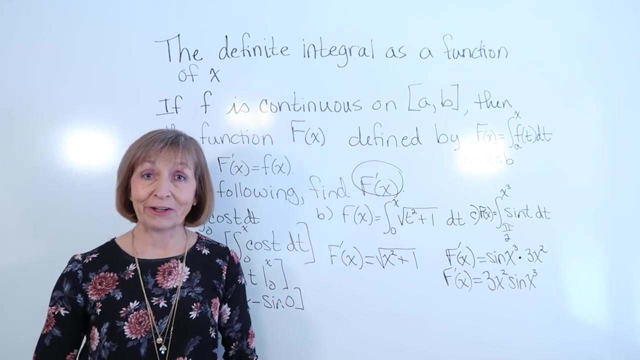 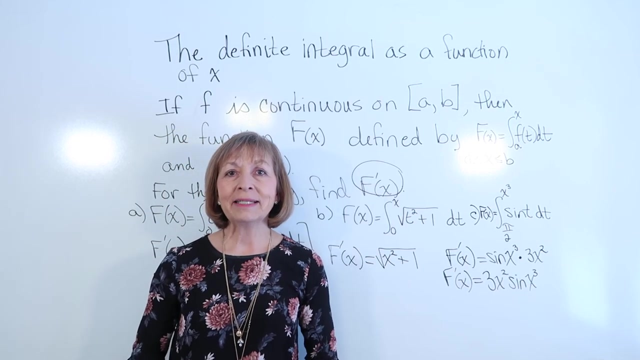 the third, And that gives you several different examples of not only evaluating function types that are defined this way, but also using that application of the second fundamental theorem of calculus to find the derivative of functions that are defined in that way. Well, thank you for watching my video and please push the like button if you found this.